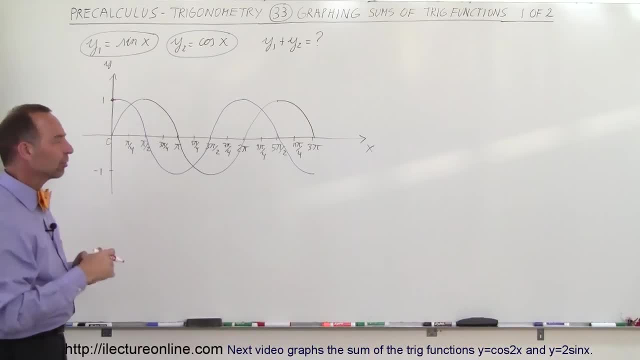 square root of 2 over 2.. So if you add them together, .707 plus .707 is about 1.4.. So I'll draw the dot right there representing a value of about 1.4.. So if you add .7 plus .7 together, we get 1.4.. 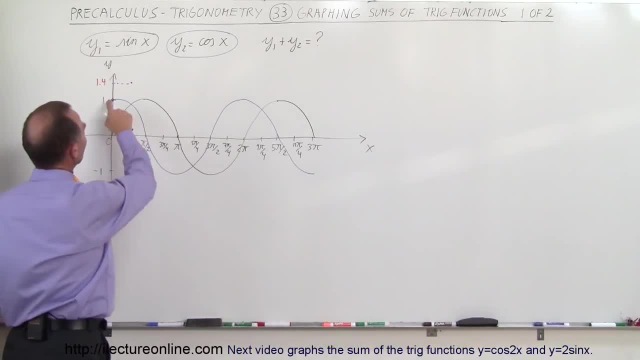 At pi over 2, at 90 degrees, you can see that the cosine is 0 and the sine is 1, so we're back over to this point right there. At 3pi over 4, notice that the sine is plus .7 and the cosine is minus .7.. They have the same value of 0.. 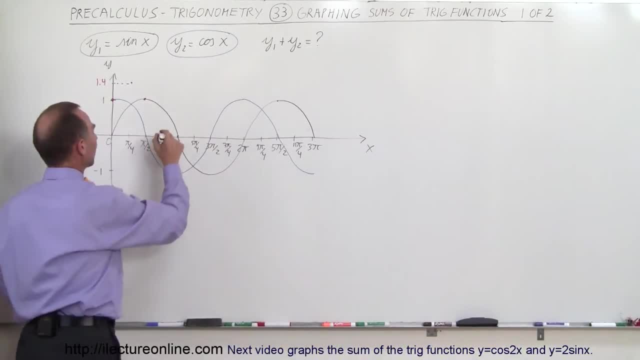 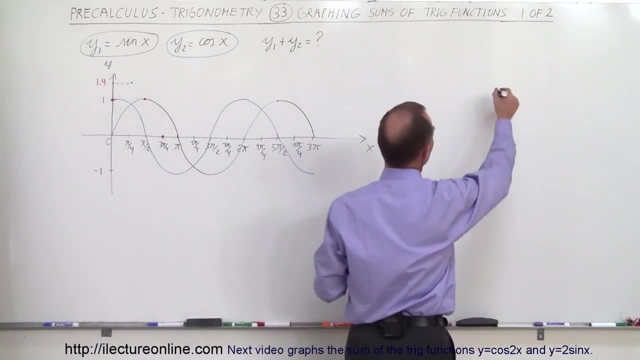 value, but the cosine is negative and the sine is positive. So that means that when I add these together I get a zero value. So if this seems a little odd to you again, you can go to the unit circle. So if you have the unit circle right here, notice that at 3 pi over 4, which is 135 degrees. 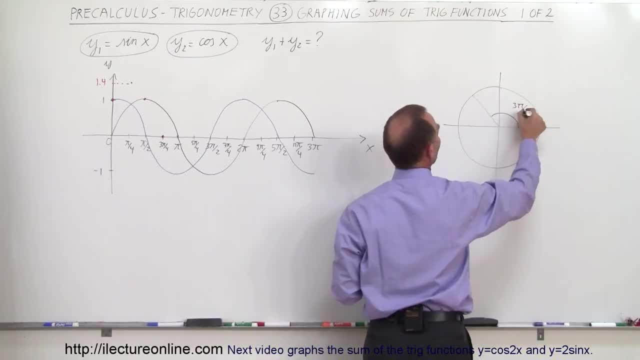 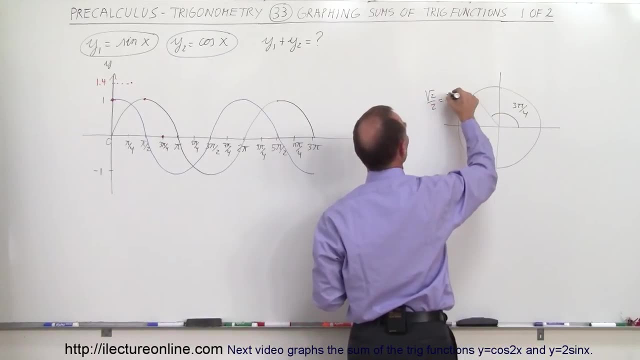 so that gives you an angle of 3 pi over 4, 3 pi divided by 4.. Notice that the y value is equal to the square root of 2 over 2, which is equal to 0.707,, and the x value is minus the square root of. 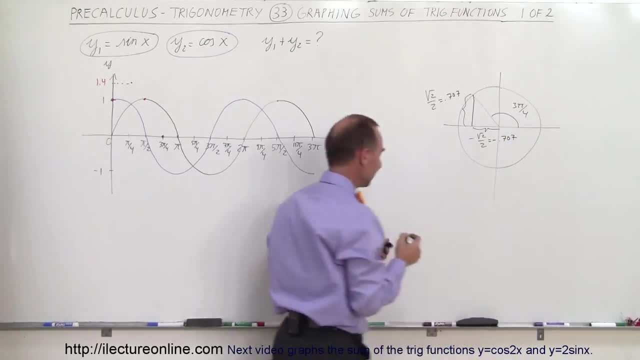 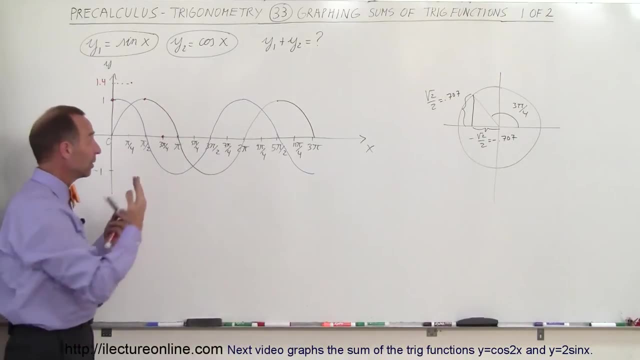 2 over 2, which is equal to minus 0.707.. So that's indicated right here. at this point where we have the positive value for the sine and the negative value for the cosine, When you add them together you get zero. Over here at pi see that the sine is zero and the cosine is negative: 1,. 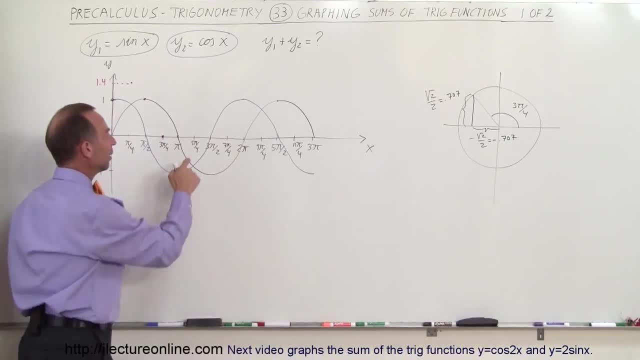 which gives you a value of negative 1.. And over here, at 4, 5, pi over 4,, both the cosine and the sine are at 45 degrees, or a better way to say it is that the value of the sine and the cosine is minus square root of 2 over 2, or 0.707, but in a negative. 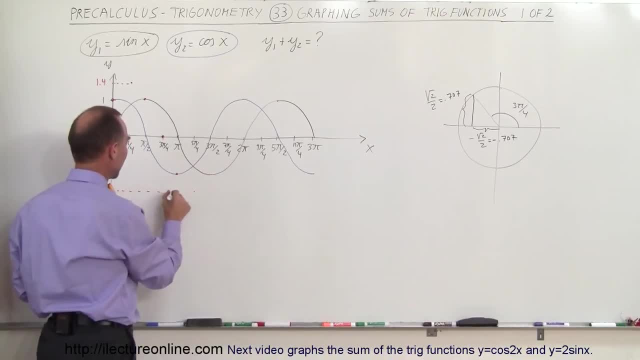 direction. So add them both together and you get a value of about minus 1.4 right there. And then, coming back over here, 3 pi over 2, notice that the cosine is zero and the sine is negative 1.. 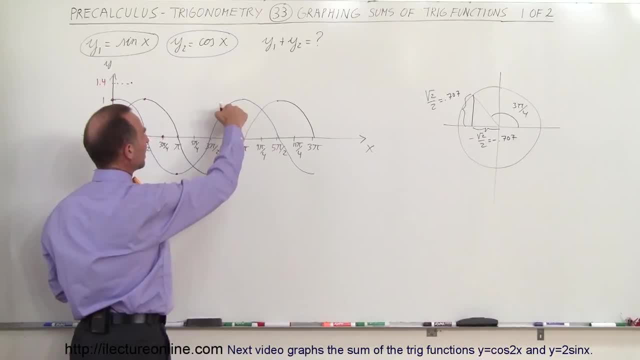 So add them together, you get negative 1. Over here. what we call the cosine is negative 1. Plus 0.7, and the sine is minus 0.7, so they cancel each other out. you get zero Over here. 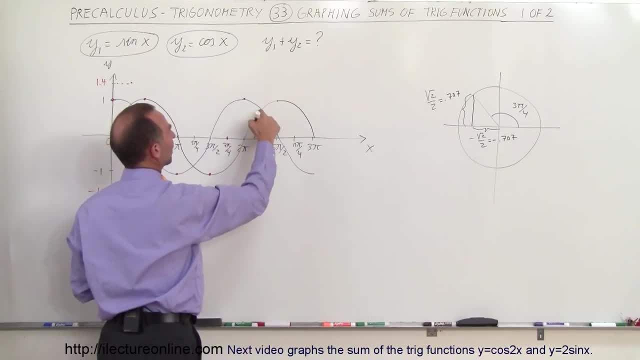 you can see that the sine is zero and the cosine is 1.. Over here they're both 0.707, so they both add up to about 1.4.. Here we have 1 plus 0, gives you 1.. And here they cancel each. 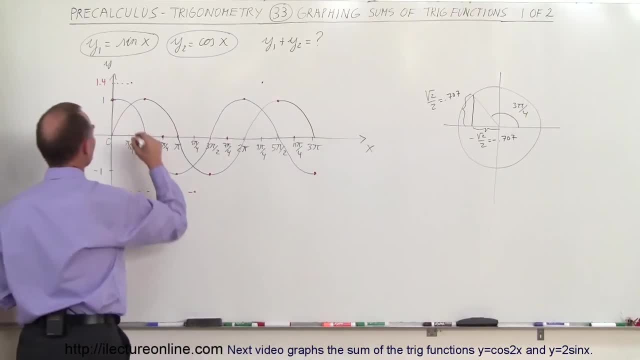 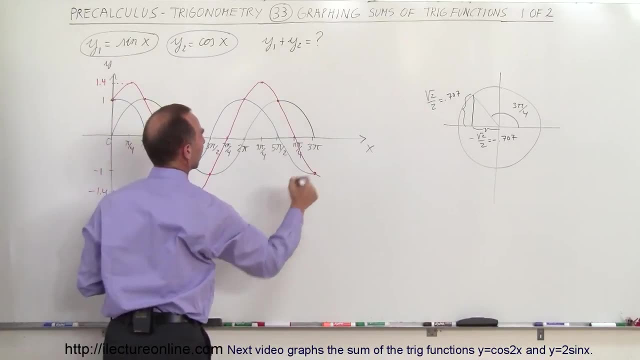 other out again and over here it is negative 1. So when we connect all the red dots, we get something that looks like this, Like that, And so that would be the sum of the cosine and the sine added together. Some of the details: 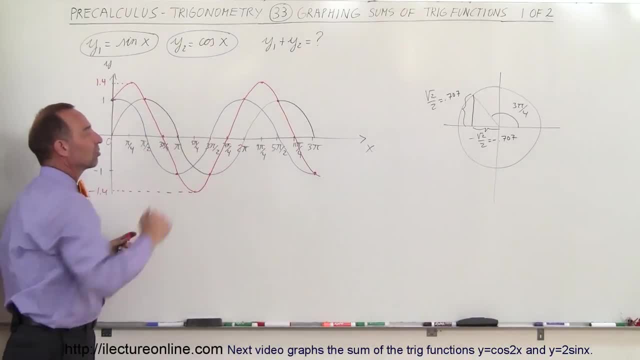 may be missing, but at least we have the general form of that summation, And so that would be the sum of those two, and that's how we do that. Now, if you're not sure how to do it like this, what you can also do is put up a table of values. You can put up the angle. 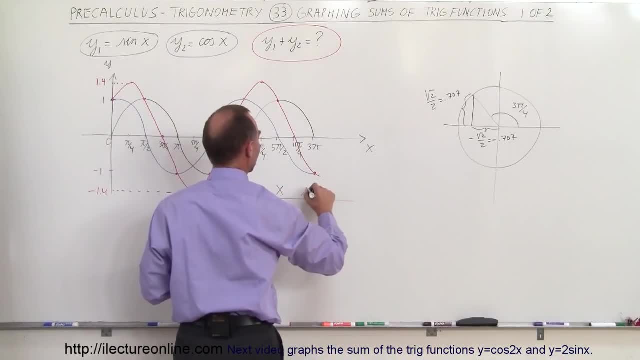 x. Then you can go, then you can say: what is the sine of x, what is the cosine of x, and then you simply sum them together. And then you can go back over here. you get a sum them together. Sum So, when x is equal to 0,, the sine is 0,, the cosine is 1, the sum is 1.. 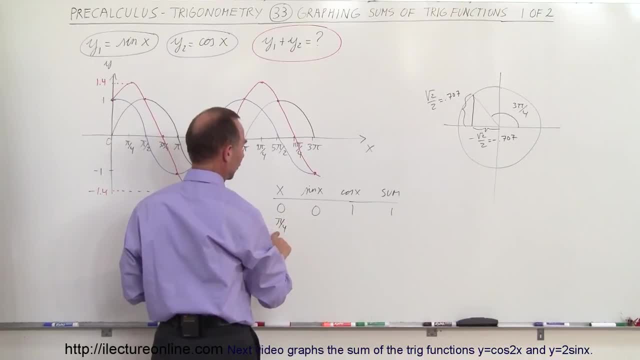 When x is equal to pi over 4, that's 45 degrees right, 45 degrees. The sine of x is the square root of 2 over 2, which is 0.7.. The cosine of x, square root of 2 over 2, which is 0.7.. Add it together. 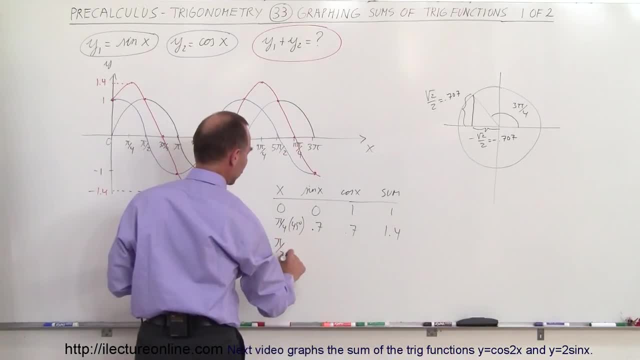 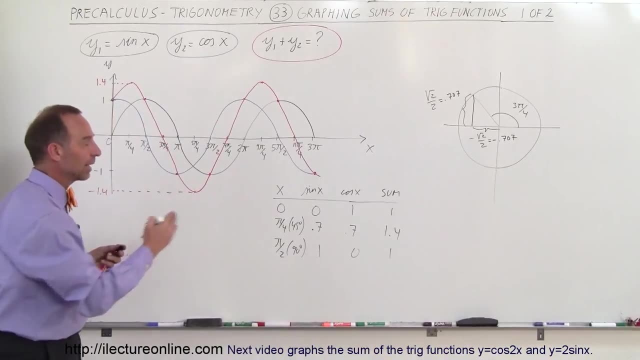 you get 1.4.. At 90 degrees, pi over 2,, 90 degrees, the sine is equal to 1,. the cosine is equal to 0. Add it together, you get 1.. And so you can do the same thing like that, and you simply will get. 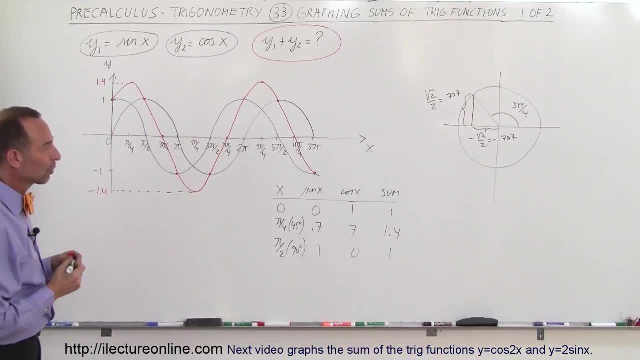 the overall shape of the summation of the two trigonometric functions And that's how we do that. So that was a simple example. On the next video I'll do a little bit more complicated example with a different value for k and a different value for the angle, and you'll see.